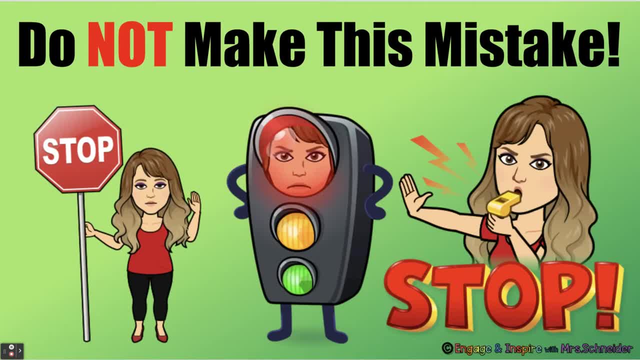 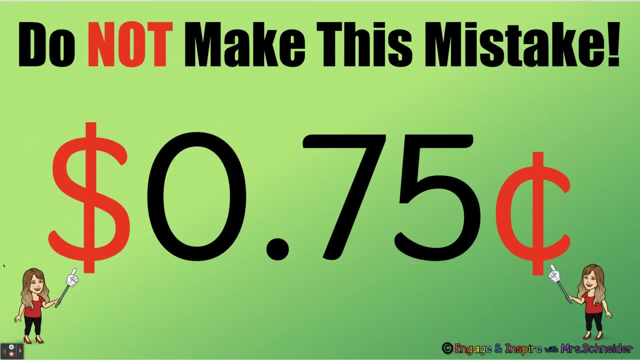 Do not make this mistake, Stop, stop. Do not make this mistake. What do you see wrong with this picture? What's wrong with it? It says 75 cents. What do you see wrong with this picture? It says 75 cents. 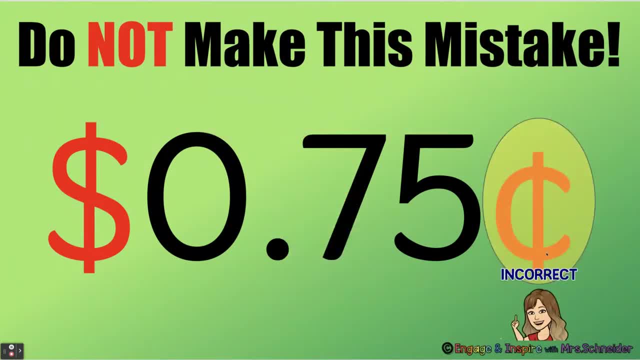 This is incorrect. We don't use both signs at the same time. You have to choose one or the other. Okay, So this would be one way to write: 75 cents: Dollar sign: zero dollars, decimal point: 75 cents. 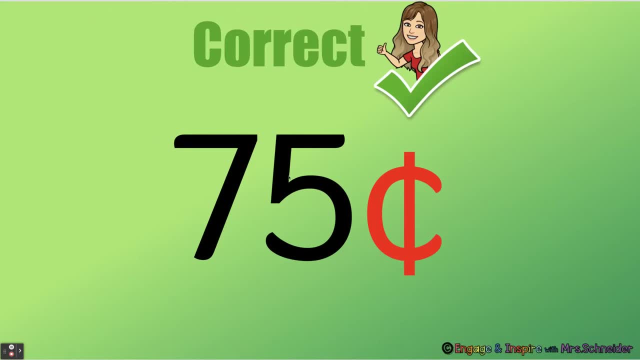 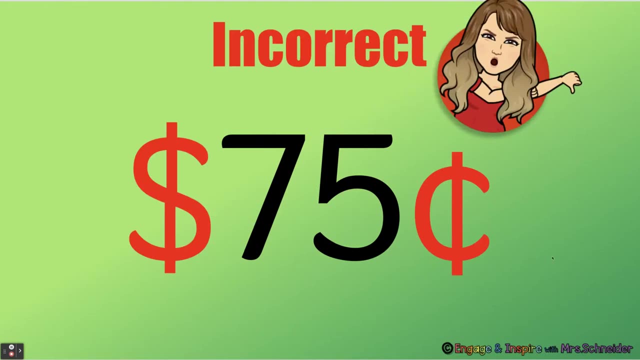 No cent sign. This is a correct way to write 75 cents. if you use just the cent sign, This is incorrect. This says $75 cents. That doesn't make any sense, does it? No, do not write it that way. 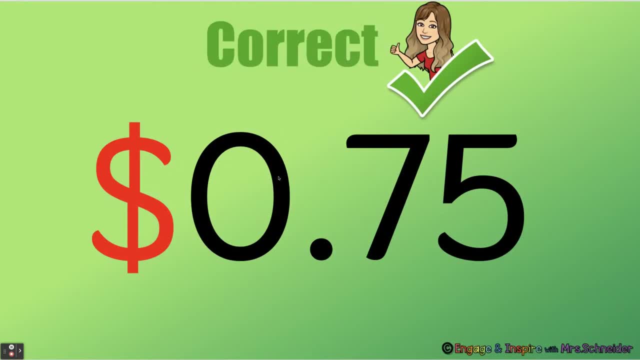 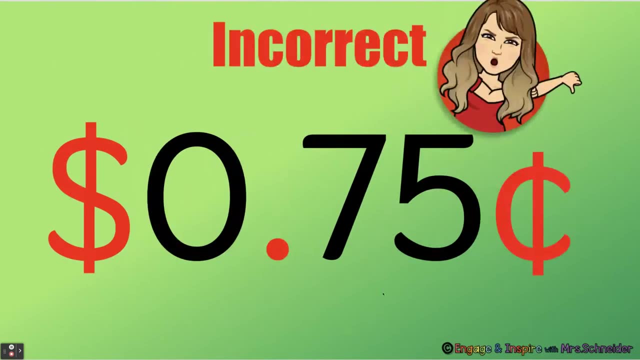 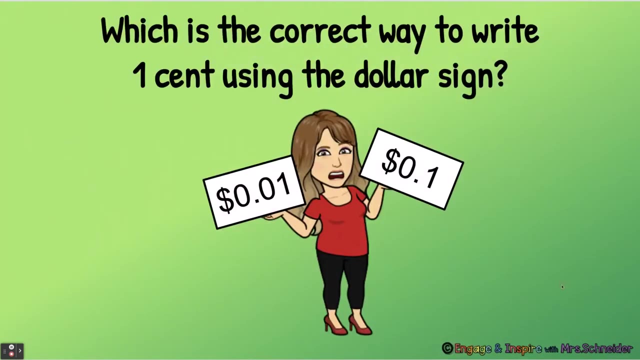 We cannot use both signs. This is a correct way to write 75 cents. Zero dollars. decimal point: 75 cents. This is incorrect. See how they put both signs there. That is wrong, Which is the correct way to write one cent using the dollar sign. 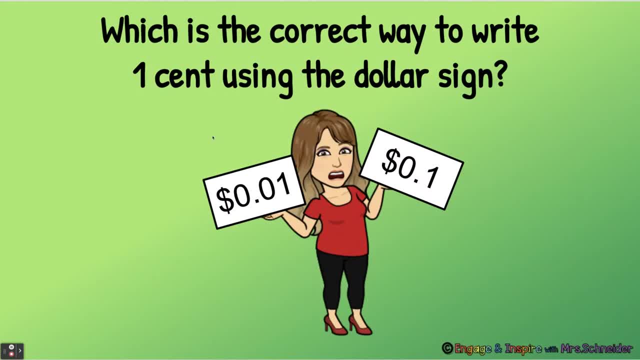 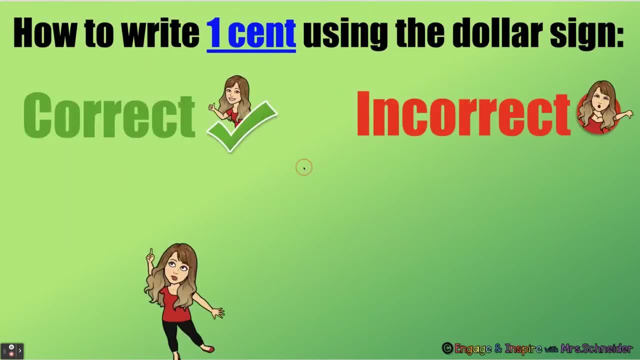 This is a mistake that lots of second graders make When we write one cent or two cents. let's see how we do that. So the correct way to write one cent is like this: Zero dollars, decimal point zero, one cents. 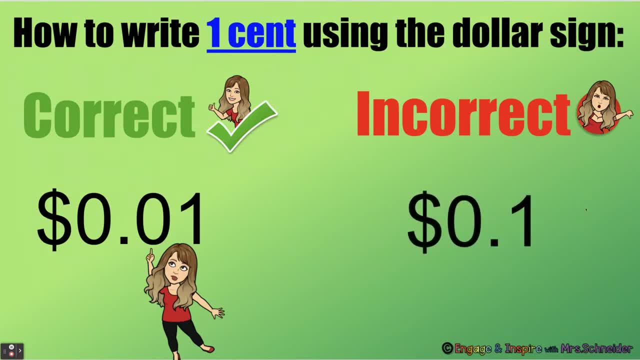 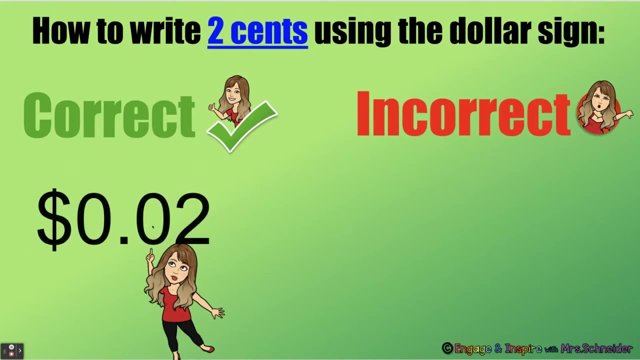 It's incorrect to put decimal point one, because this would be the same as if there was a 10 right here, So that one is wrong. The correct way to write one cent would be decimal point zero one, And the correct way to write two cents is decimal point zero two. 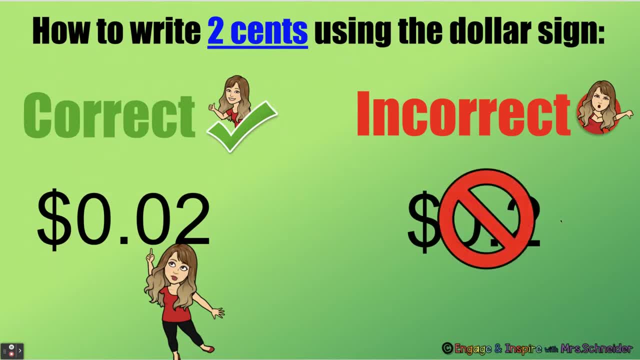 Okay, not decimal point two. That would be the same as 20.. That's wrong. And the correct way to write three cents is zero three. The correct way to write four cents is zero four, Not decimal point four, because that would mean 40.. 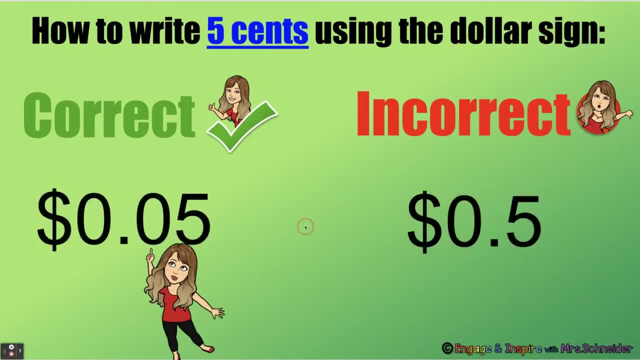 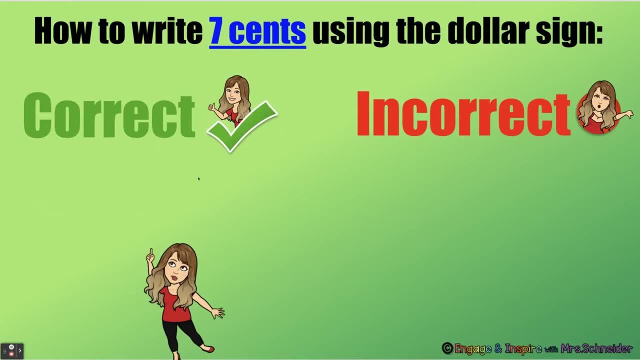 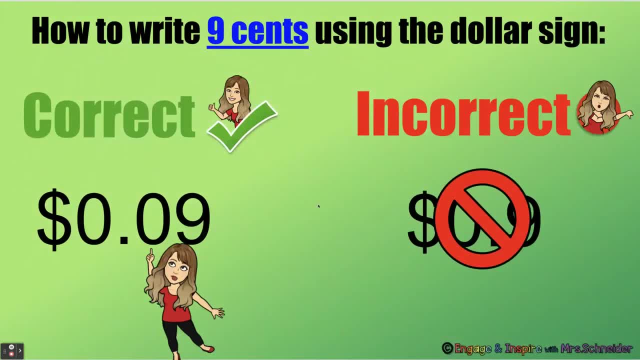 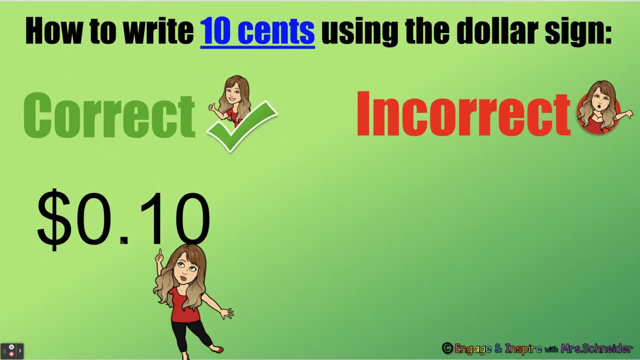 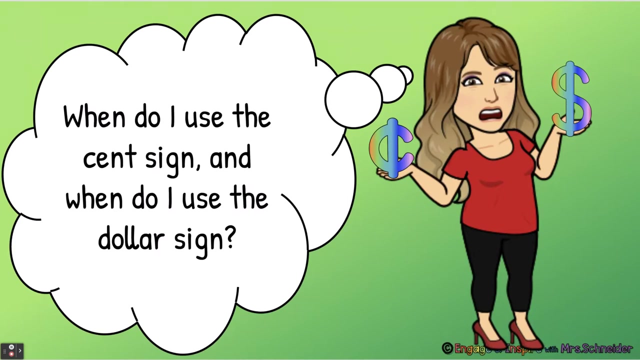 The correct way to write nine cents is zero nine And the correct way to write ten cents is decimal point one. zero for ten, Decimal point ten. That's the correct way to write ten cents, Not like this. When do I use the cent sign and when do I use the dollar sign? 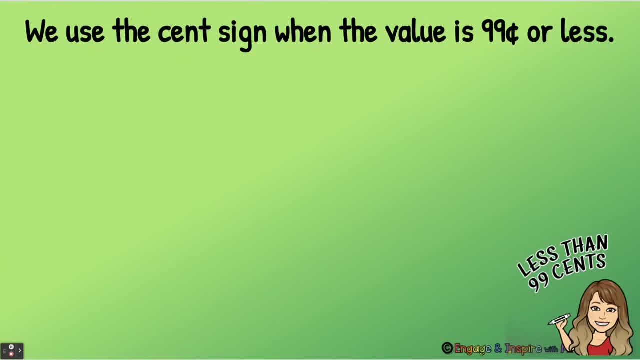 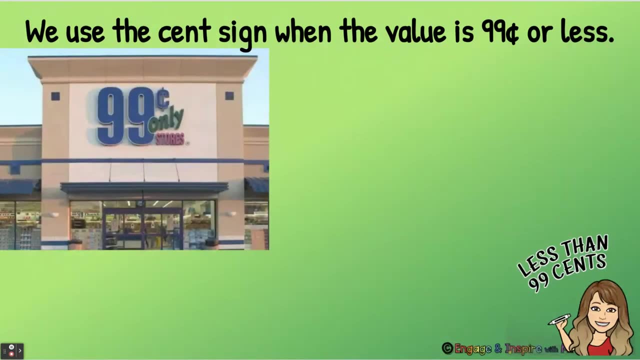 Oh, good question. We use the cent sign when the value of the dollar is zero. The value is 99 cents or less. Think about it: 99-cent store, 50-cent store. See the cent sign. See the cent sign. 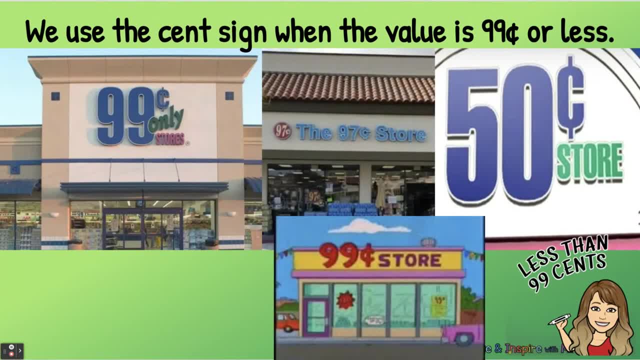 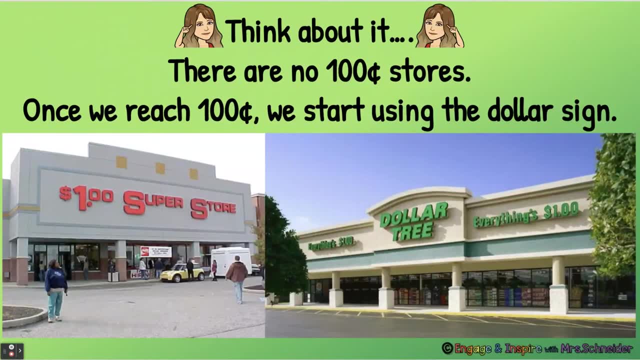 97-cent store, 99-cent store, 33-cent store. Think about it: There are no 100-cent stores. Once we reach 100 cents, we start using the dollar sign. Remember: 100 cents is the same as one dollar. 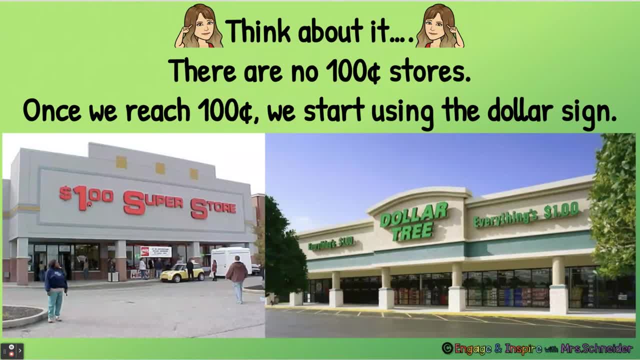 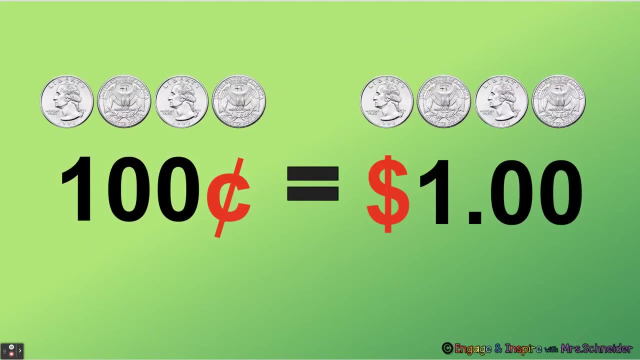 So then we put dollar sign one decimal point and zero cents And here at the dollar tree we have dollar sign one decimal point, zero cents. So 100 cents can be written this way using the dollar sign. Dollar sign one decimal point, zero, zero. 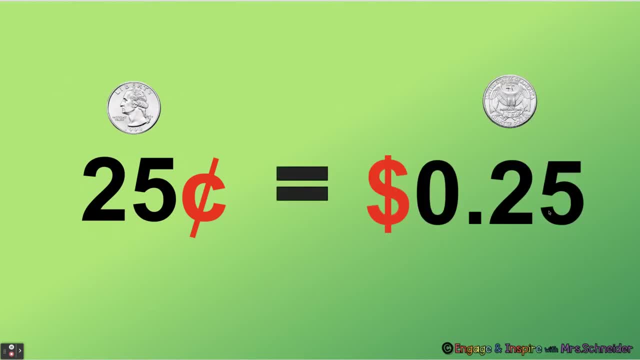 And 25 cents can be written like this: Dollar sign: zero, decimal point 25.. This says 25 cents and this says 25 cents. 50 cents can be written like this: Dollar sign: zero dollars, decimal point 50 cents. 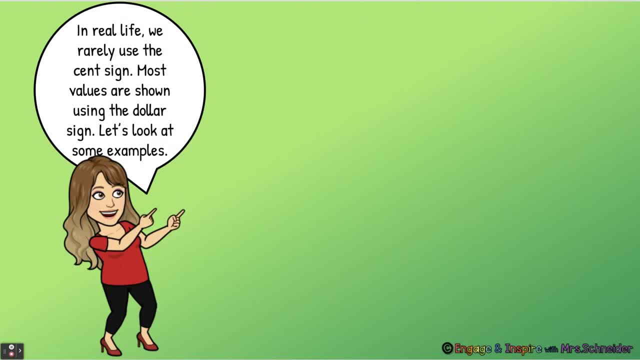 In real life we rarely use the cent sign. Most values are shown using the dollar sign. Let's look at some examples. So this wood butterfly that you can paint from Walmart is 77 cents. See how it's shown with the dollar sign, not the cent sign. 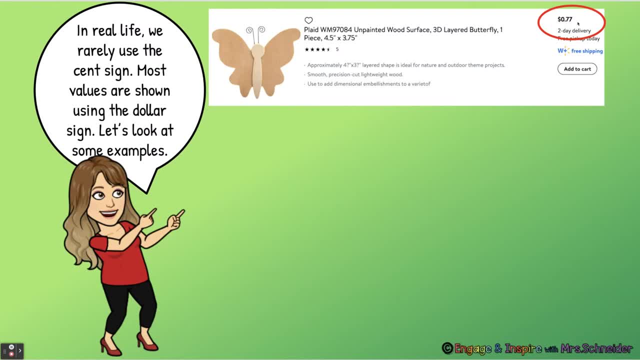 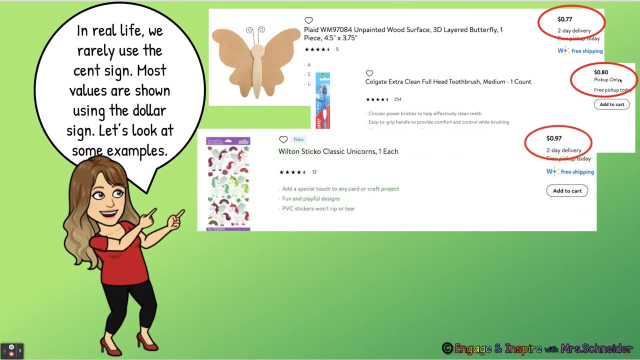 It says zero dollars dot 77 cents And this Colgate toothbrush is 80 cents. You see there No dollars, There's just 80 cents. but it's using the dollar sign, not the cent sign, And these beautiful unicorn stickers are 97 cents. 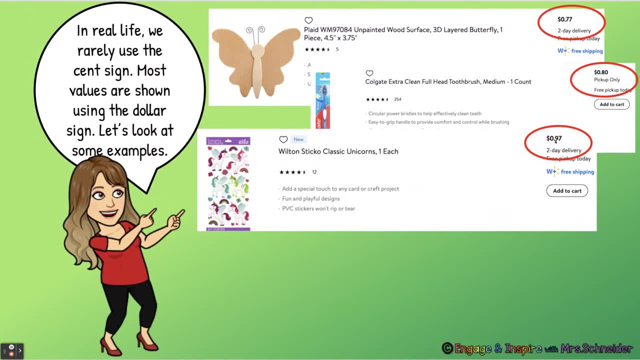 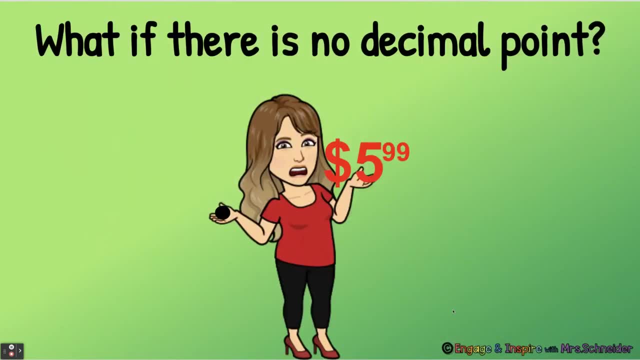 And that's using the dollar sign Zero dollars. decimal point: 97 cents, And this Hot Wheel is 99 cents. What if there is no decimal point? Does this number say 590?? No, it doesn't. Does it say 599, or does it say $5.99?? 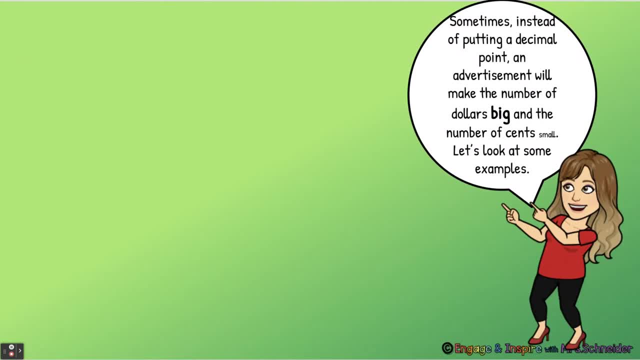 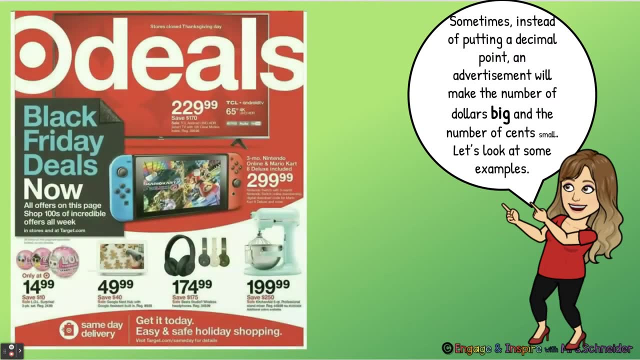 Sometimes, instead of putting a decimal point, an advertisement will make the number of dollars big and the number of cents small. Let's look at some examples. Here we see a Target ad. Let's look at the prices on here. So this Nintendo Switch is $299.99. 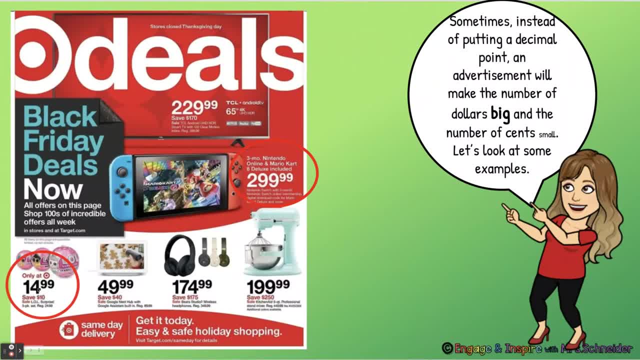 $299.99.. $299.99.. And these LOL dolls are $14.99.. And this Google Nest Hub is $49.99.. And these Beats headphones are $174.99.. And this beautiful mixer is $199.99. 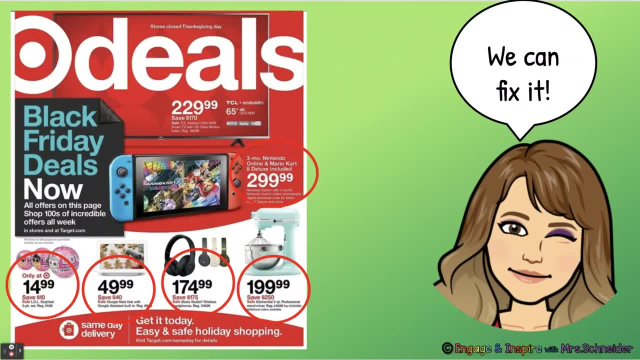 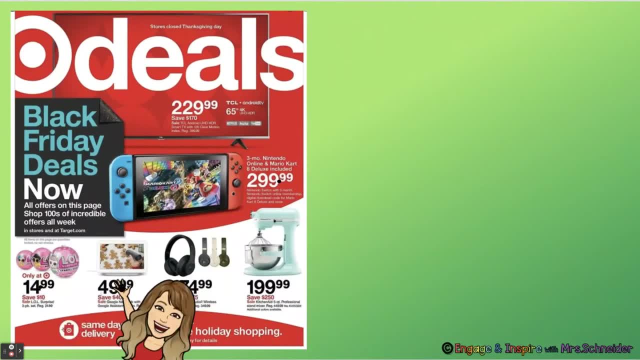 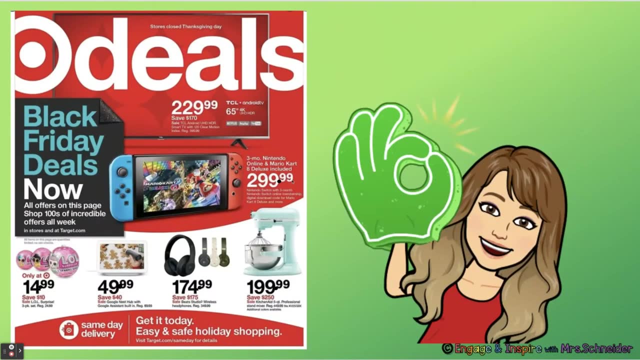 But we can fix it with decimal points, Because we know that the decimal point is going to separate the dollars from the cents. Here we go, Boom Boom, Boom, Boom, Boom Boom. There we go. We've separated the dollars from the cents with our decimal point. 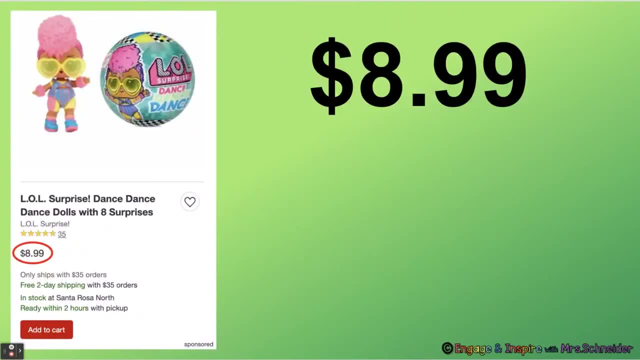 Let's practice reading some prices of toys out loud. So a lot of students just say $8.99.. We need to know that this is $8.99. And this is $99.99.. So when you yell out the answer, I want you to tell me how many dollars and then how many. 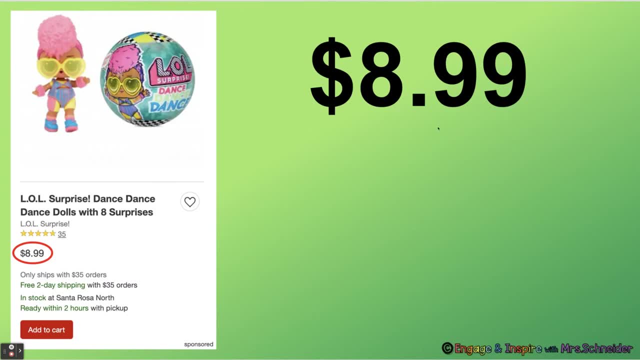 cents. Okay, You ready, I'll do this one. This, LOL, is $8.99.. See $8.99.. Good, Okay, What's this one? How much is this? Ryan's World, Mystery Adventure, Playset egg. How many dollars and how many cents? 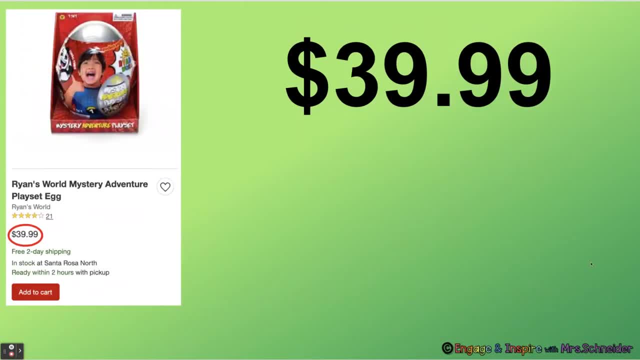 $8.99.. $8.99. Good. Okay, What's this one? How much is this? Ryan's World Mystery Adventure Playset egg. How many dollars and how many cents? $8.99. Good, How about this one? 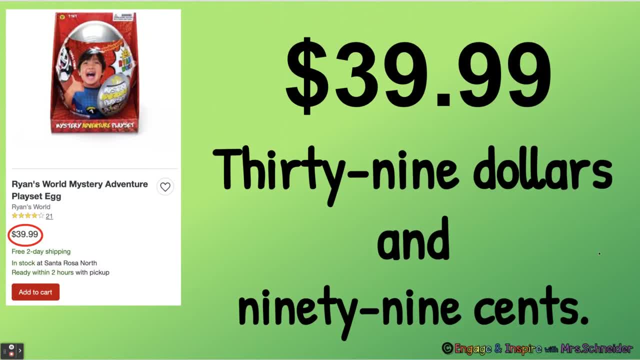 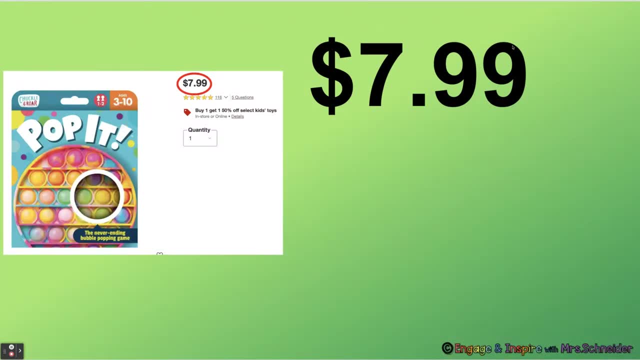 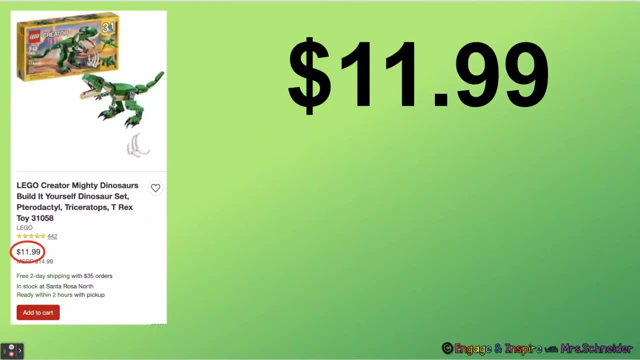 $8.99.. $8.99.. Good job. What about this one? How much is this pop-it? This pop-it is $7.99.. How much is this Lego dinosaur? It's $11.99.. Good job. 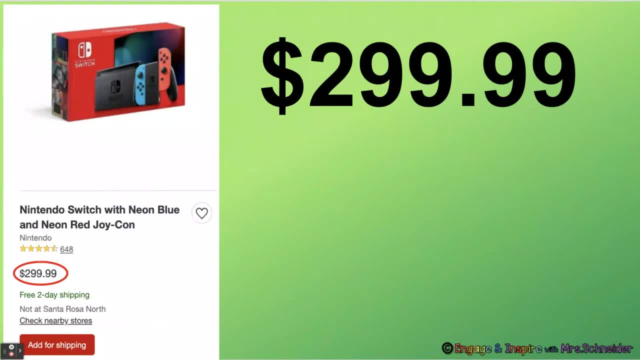 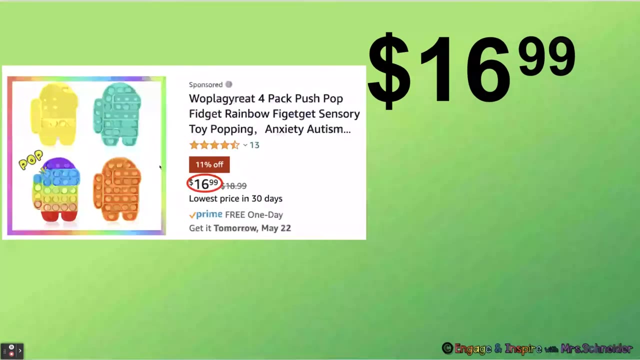 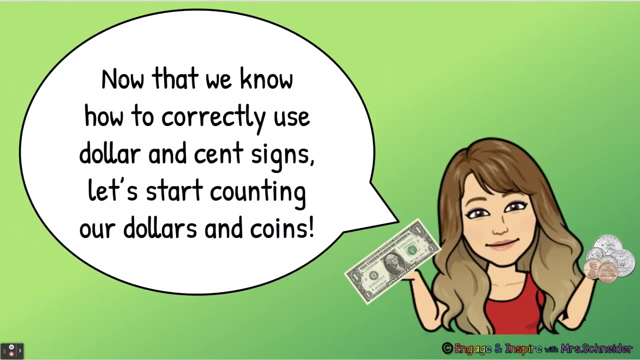 Good job. Ooh, how about this Nintendo Switch? That's pretty expensive. $299.99.. Good job. And how much are these Among Us Pop-Its? $16.99.. Good job, Now that we know how to correctly use dollar and cent signs. 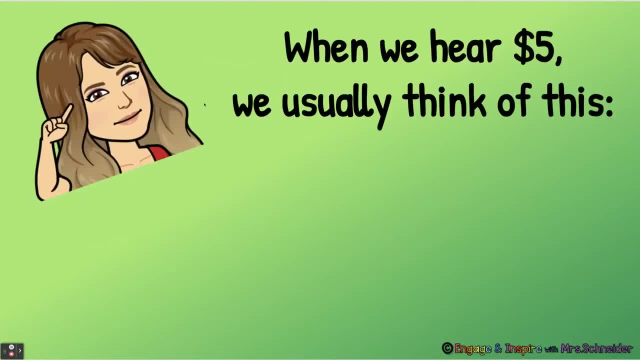 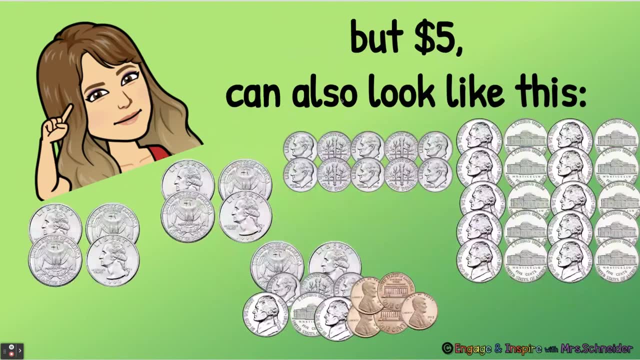 let's start counting our dollars and coins. When we hear $5, we usually think of this, But $5 can also look like this. Look at all that change. See, here's a dollar. Four quarters is a dollar. So $1, $2,, $3.. 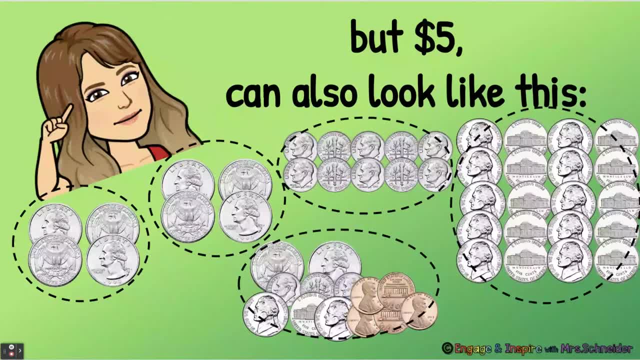 $4, $5.. So see, four quarters is a dollar. Ten dimes is a quarter. So see, four quarters is a dollar. Ten dimes is a dollar. Twenty nickels is a dollar And a whole mix of change can be a dollar. 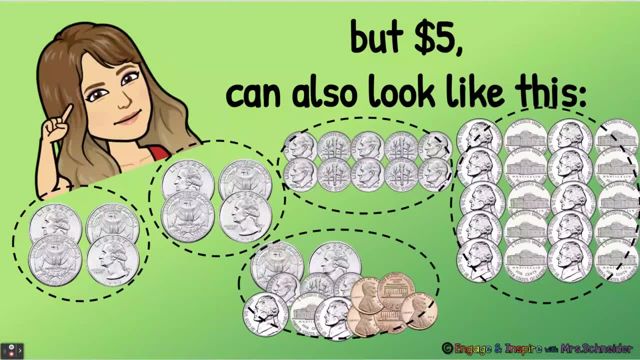 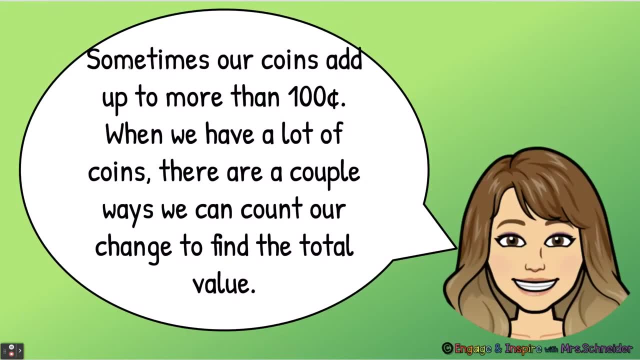 And it can add up to $5 altogether. One, two, three, four, five. Now you might want to trade for a $5 bill if you had all of this change. Sometimes our coins add up to more than $0.01.. 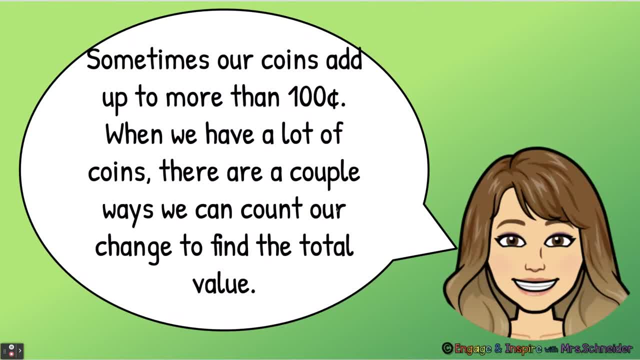 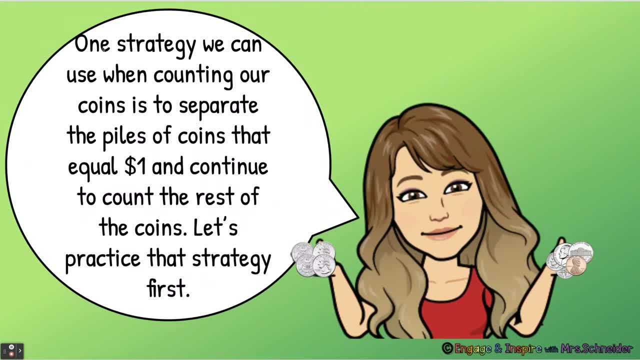 When we have a lot of coins, there are a couple ways we can count our change to find the total value. One strategy we can use when counting our coins is to separate the piles of coins that equal $1 and continue to count the rest of the coins. 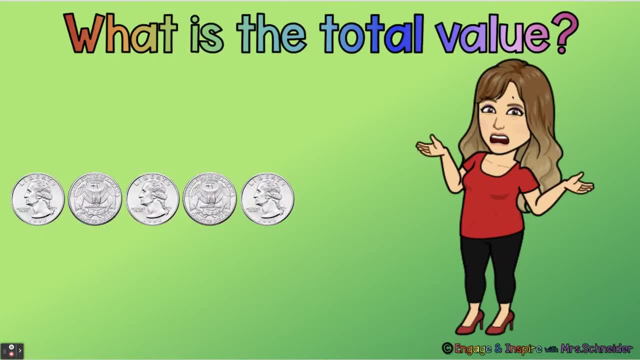 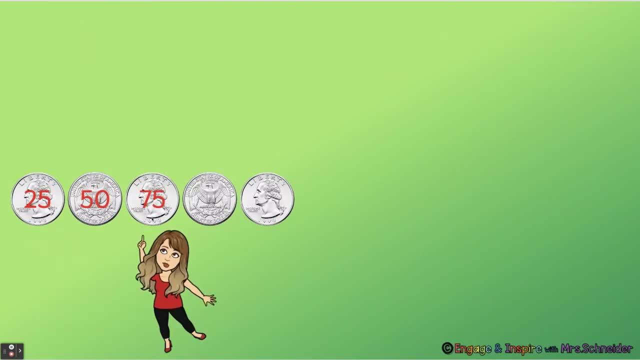 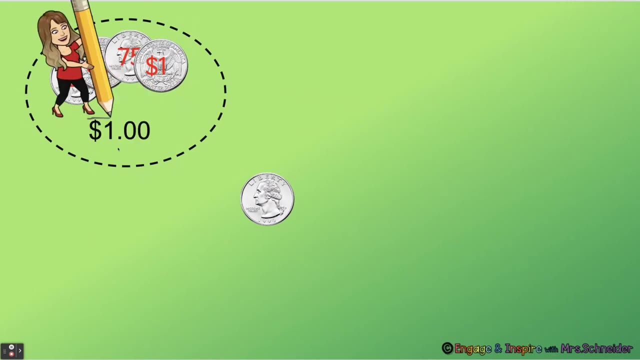 Let's practice that strategy first. What is the total value? I don't know. Let's count 25,, 50,, 75, $1.. All right, Now we can take that dollar and put it in a little pile by itself, so we know that that pile is $1.. 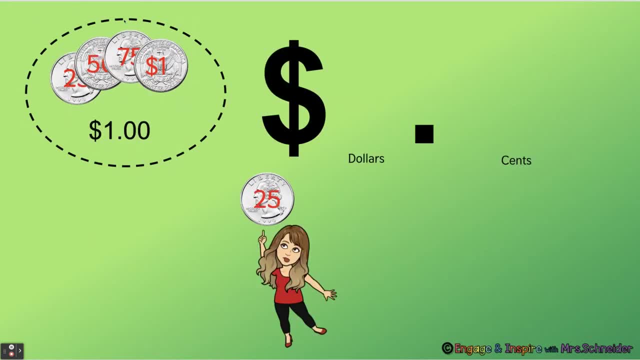 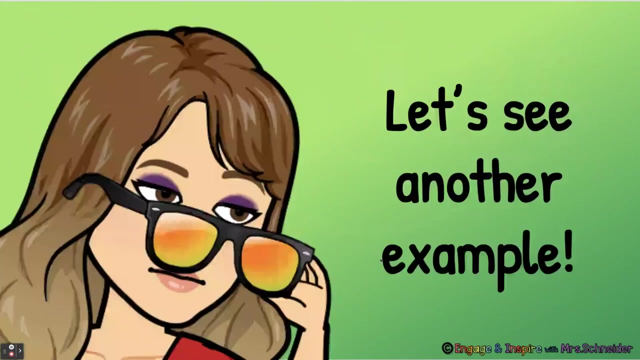 Good, So we're going to. Okay, So we have $1.. And how many cents do we have left? We have $0.25.. So our total value is $1.20.. Okay, $0.25.. Let's see another example. 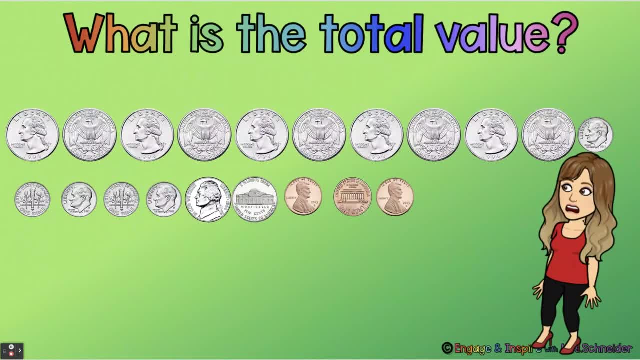 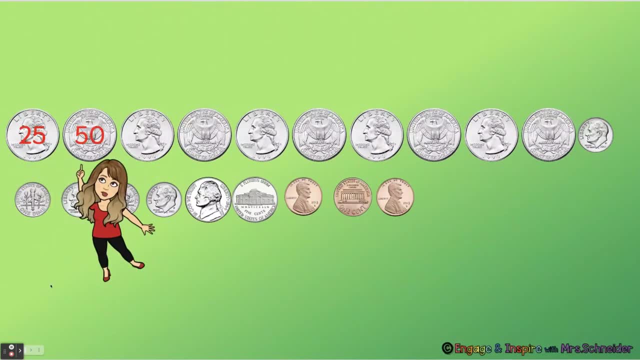 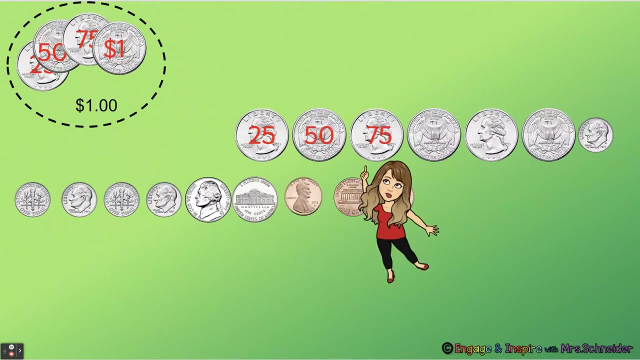 What is the total value? She looks scared. huh, That's a lot of coins. Let's count and find out: 25,, 50,, 75,, $1.. Put that in a pile: $1.. 25,, 50,, 75,, $1. 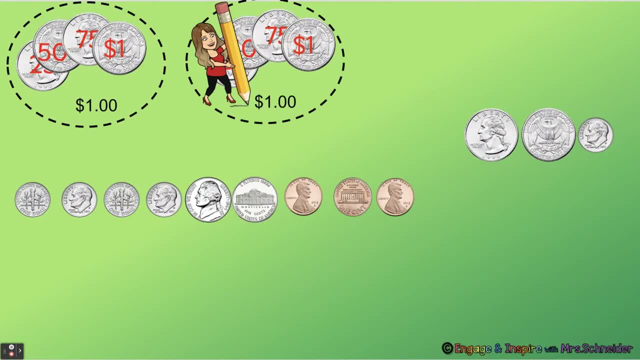 Put that in a pile. That's $1.. 25, 50.. Oh look, It was 50 plus 10 is 60.. 70, 80,, 90,, 100.. 100 cents is the same as $1.. 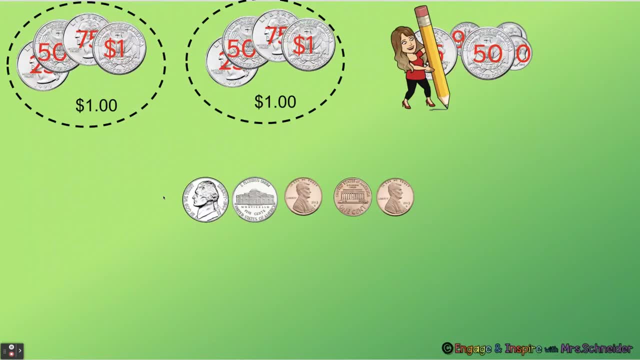 So let's gather those up and put those in a pile. All right, Now we have $3.. And we're going to keep counting our change here. So 1 nickel is 5,, 10,, 11,, 12,, 13.. 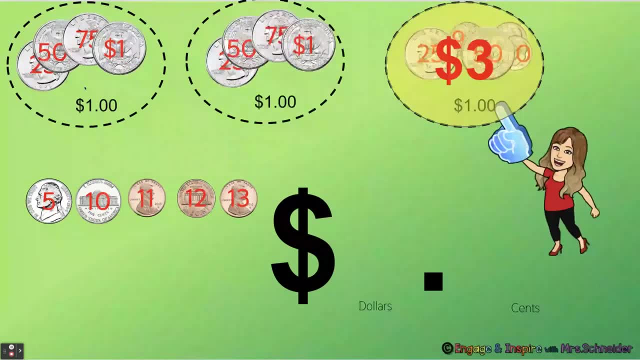 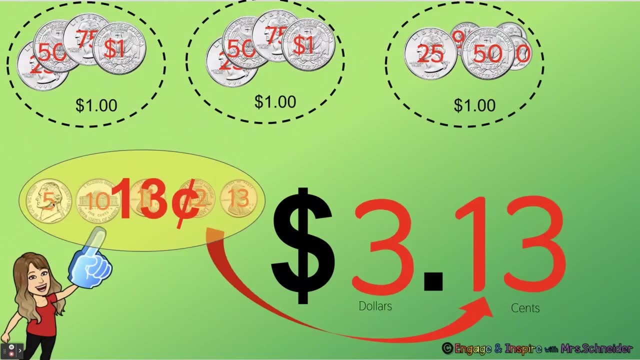 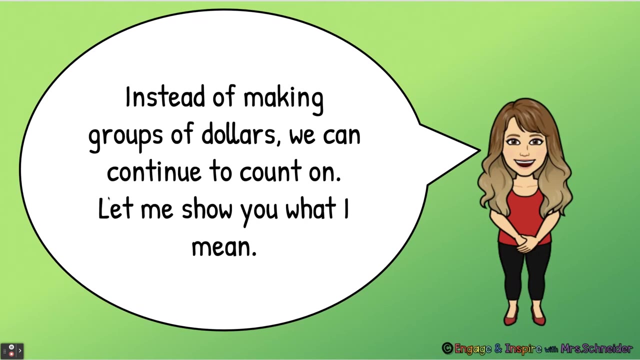 So we have 1,, 2,, $3. And how much change do we have left? And 13 cents. So $3. And 13 cents, Instead of making groups of dollars we can continue to count on. Let me show you what I mean. 25,, 50, 75, $1.. $1.25.. $1.50.. $1.60.. $1.70.. $1.50.. $1.50.. $1.80.. $1.90.. 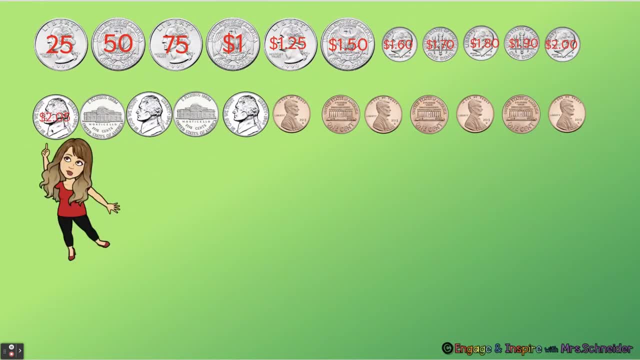 $1.90.. $2., $2.05.. $2.10.. $2.15., $2.20., $2.20., $2.25., $2.26., $2.26., $2.27.. 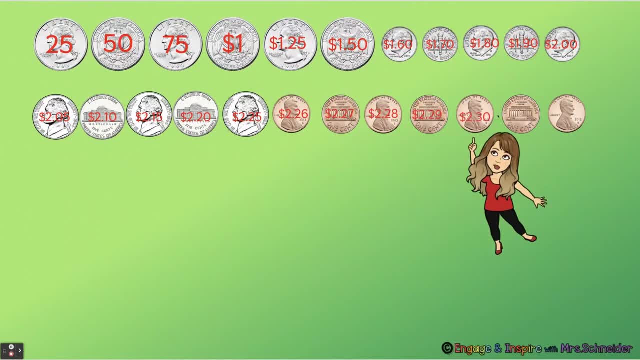 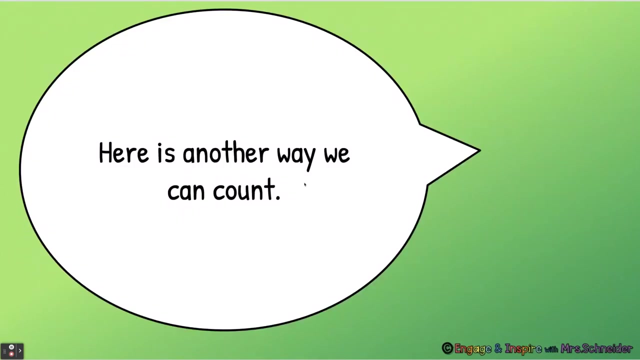 $2.28.. $2.29.. $2.30.. $2.31.. $2.32.. Ha, $2.32.. Good job. And here's another way we can count: 25,, 50,, 75,, $1. 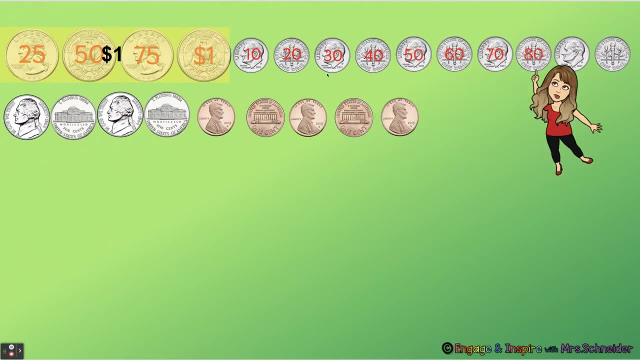 10,, 20,, 30,, 40,, 50,, 60,, 70,, 80,, 90,, 100.. That's $2.. 5,, 10,, 15,, 20,, 21,, 22,, 23,. 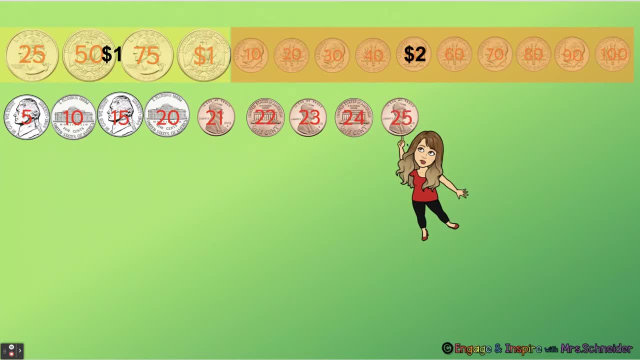 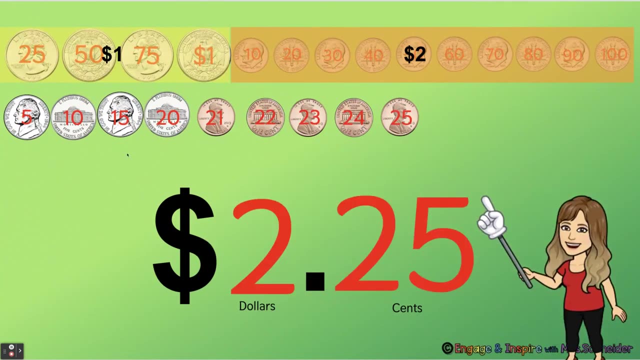 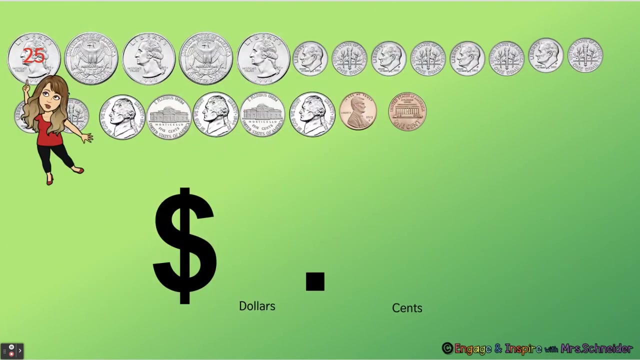 24, 25.. I know that I had $2 and 25 cents. 1,, $2, and 25 cents. Sometimes you need to rearrange your coins to make a dollar. Let's look at an example: 25,, 50,. 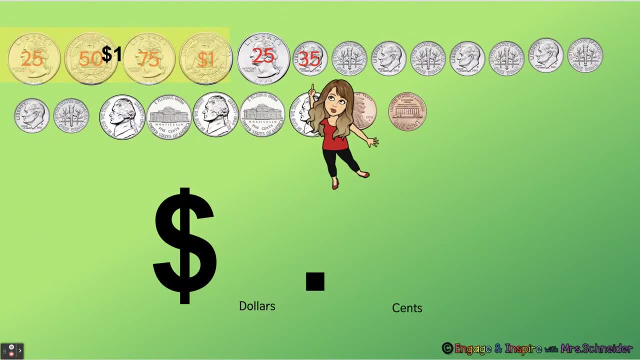 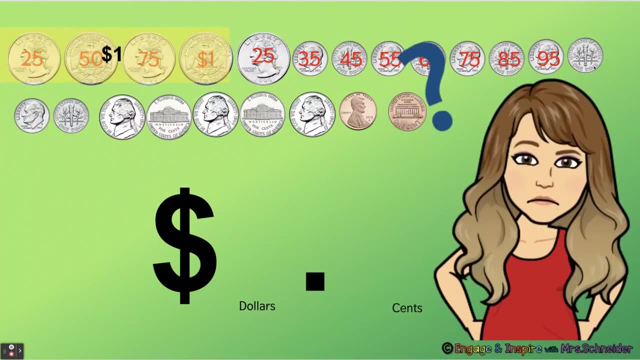 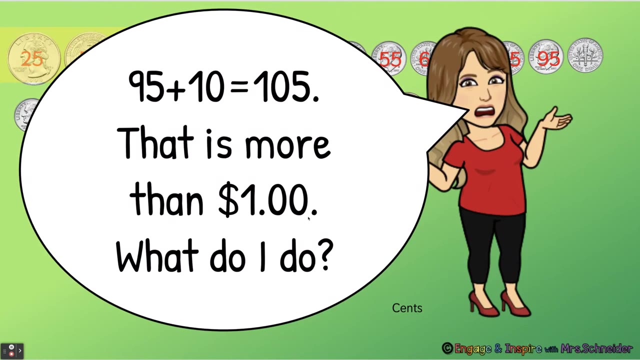 75, $1.. 25, ooh, 35,, 45,, 55,, 65,, 85,, 95,. uh-oh, 95 plus 10 is 105.. That's more than a dollar. What do I do? 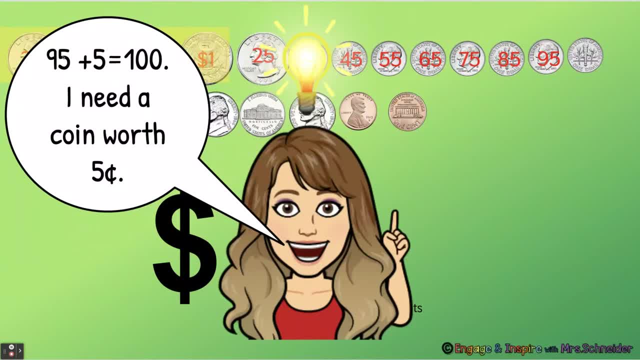 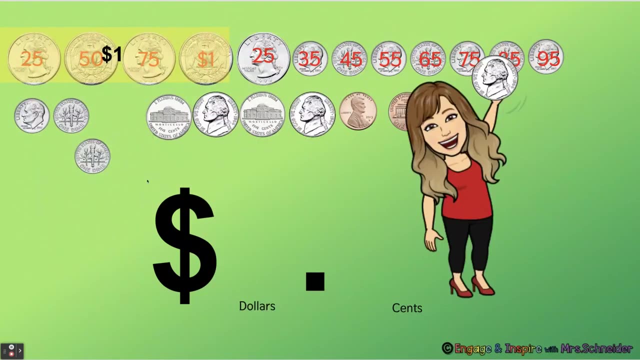 Hmm, I have an idea. Well, I know that 95 plus 5 more is 100. So I need a coin worth 5 cents. What coin is worth 5 cents? Aha, I know. So I'm going to take that dime. 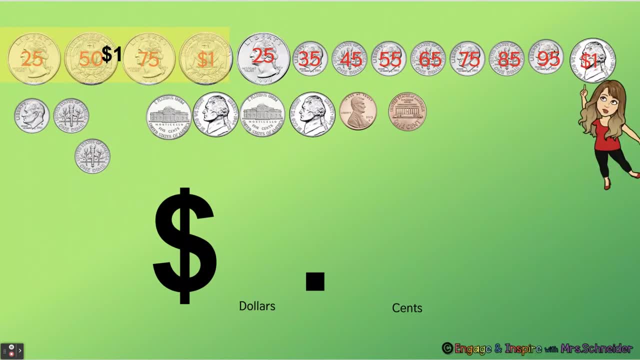 and move it down there and I'm going to put my nickel up here. There we go: 95 plus 5 is $1.. So now I have $2. And now I can count my change: 10,, 20,, 30,. 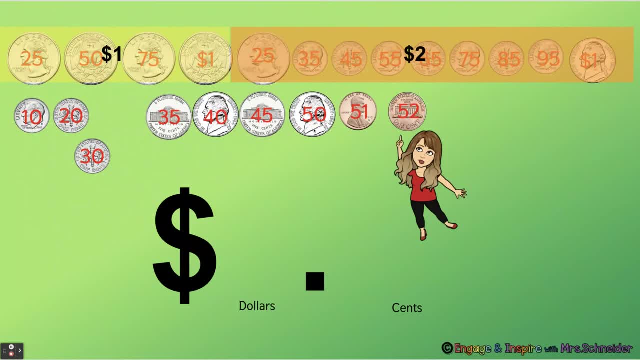 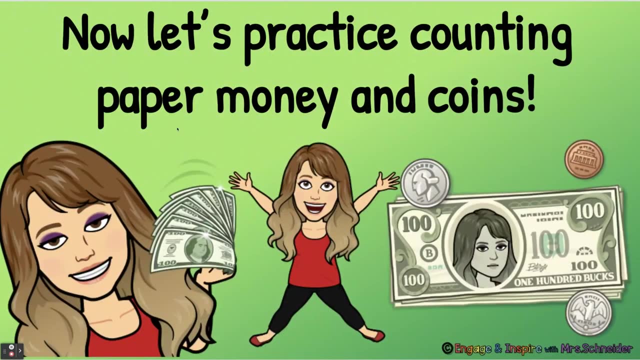 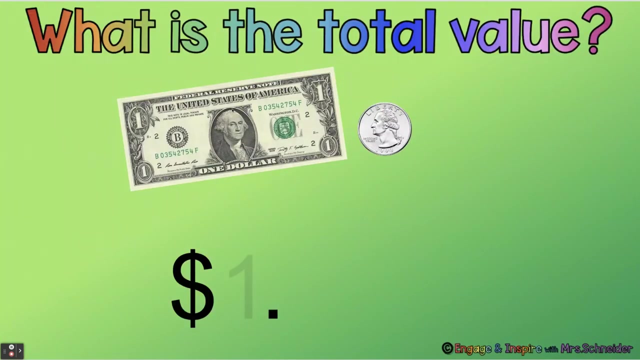 35,, 40,, 45,, 50,, 51,, 52.. So I have 1,, $2, and 52 cents. Now let's practice counting paper money and coins. What is the total value? There's $1,. 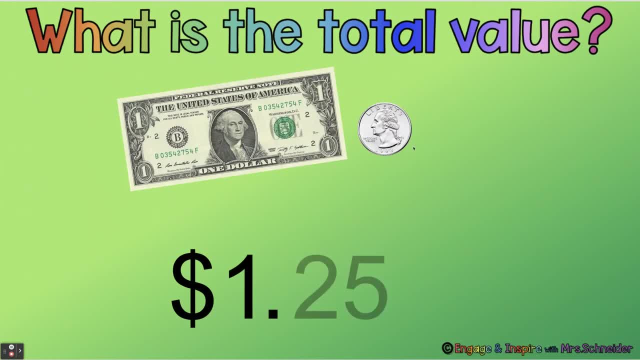 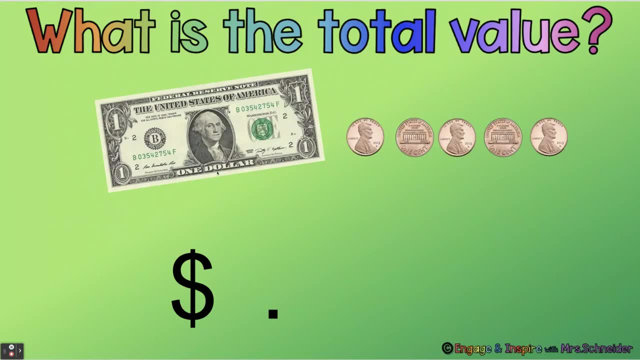 and how many cents And 25 cents, $1, and 25 cents. What's the total value here? $1, and 1,, 2,, 3,, 4,, 5 cents. Remember we're going to write 05.. 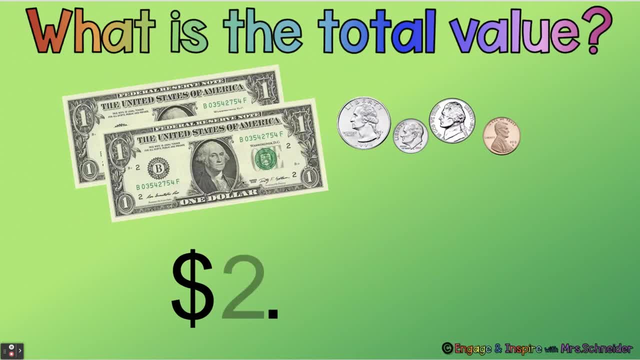 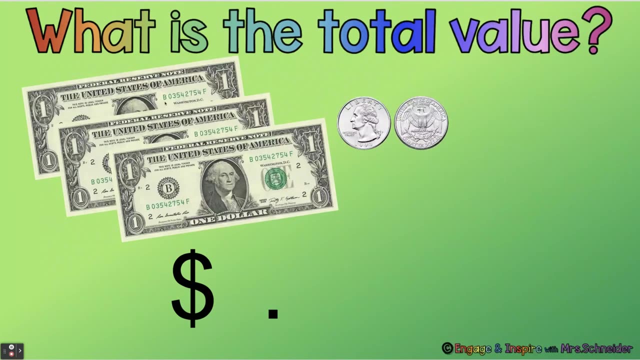 What's the value here? We have 1, $2, and 25,, 35,, 40,, 41, and 41 cents. $2, and 41 cents. What's the total value here? 1,, 2,, $3,. 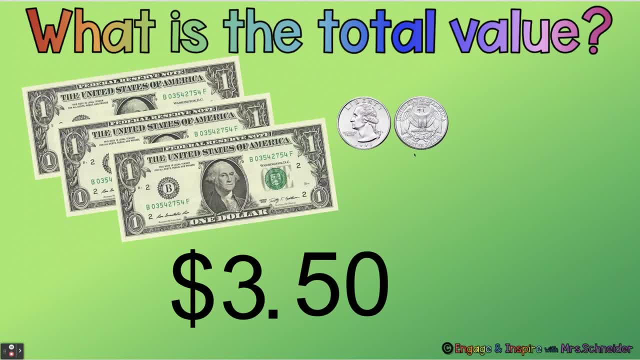 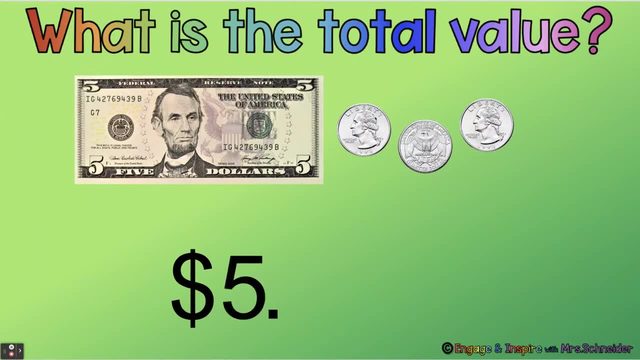 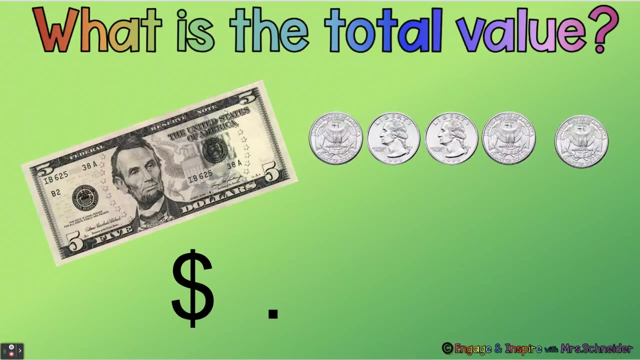 and 50 cents. 2 quarters is 50 cents. What's the value here? We have $5, and 75,, 5 cents, right? 25,, 50,, 75.. Ooh, this one's tricky. 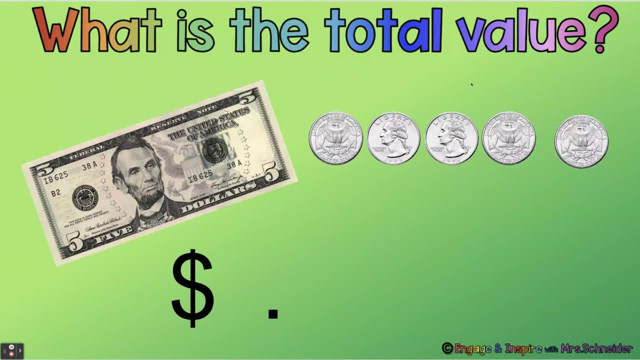 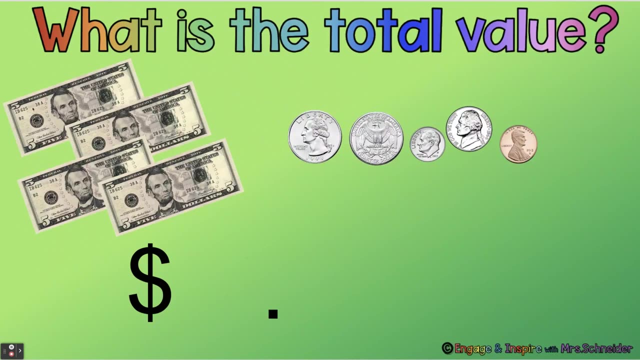 Before we start counting, look, There's 5 quarters. We know that 4 quarters is a dollar, So we have 5, 6 dollars, and how many quarters was left over? 25 cents, Good, Okay, when we have. 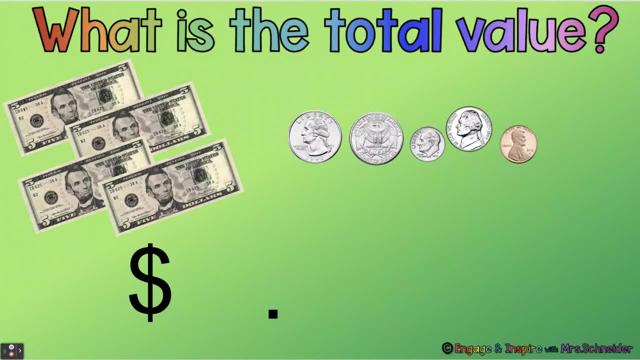 $5 bills. we can count by fives, So we have 5,, 10,, 15,, 20,, $20, and 25,, 50,, 60,, 65,, 66 cents, $20, and 66 cents. 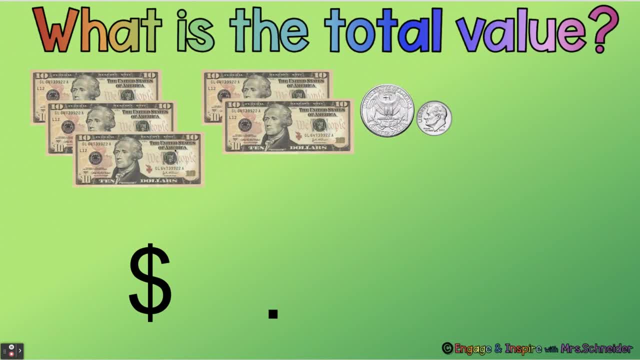 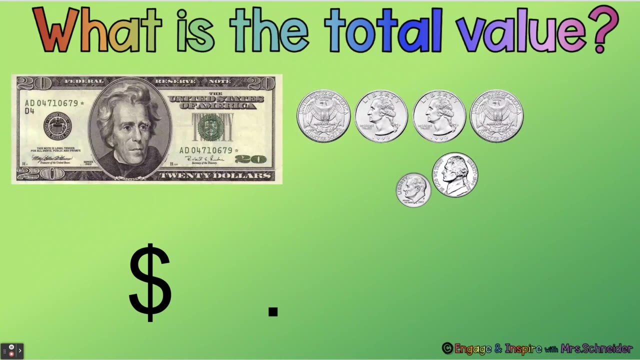 And when we have $10 bills, we can count by tens: 10,, 20,, 30,, 40,, 50. We have $50,, 55,, 35 cents. Ooh, look, A $20 bill. 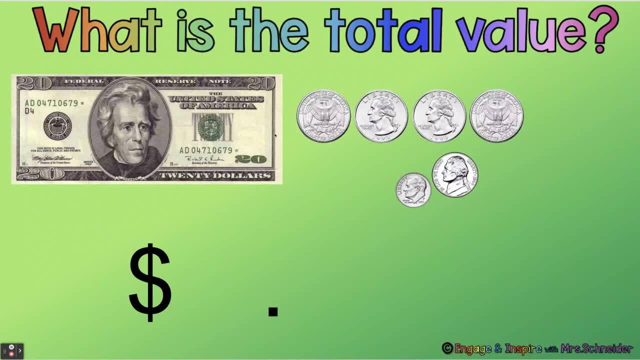 Ooh and look, There's 4 quarters here, So let's count all of our dollars before we count all of the coins. Okay, So we know this is $20, plus one more dollar would be $21.. And then 10. 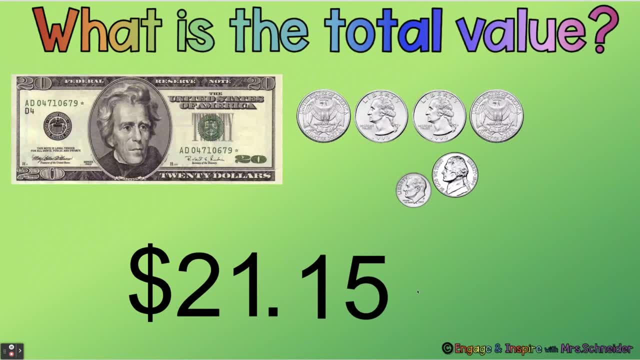 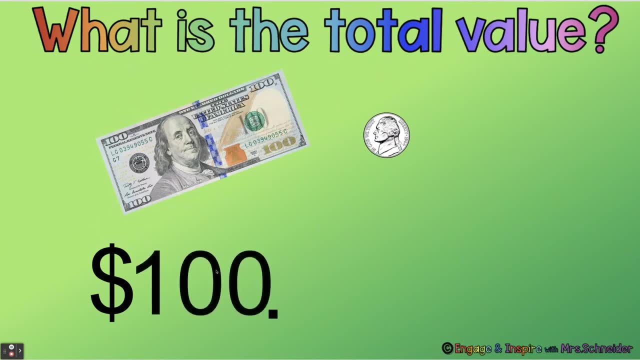 plus 5 is 15.. So $21 plus 5 is 15.. Ooh, $100.. Oh my goodness. So here we have $100.. And how many cents do we have? And 5 cents, Make sure you put 05..